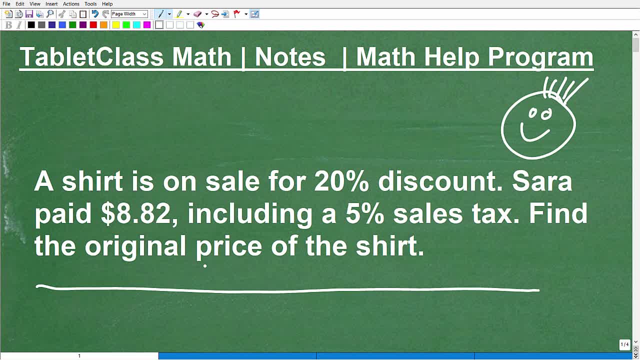 course, if you think you know how to do this problem, you should always kind of pause the video and see what you do. you kind of can put together one thing. I will state, though: in any word problem: you want to have structure, you want to have a logical set of steps that your teacher could read and be like. 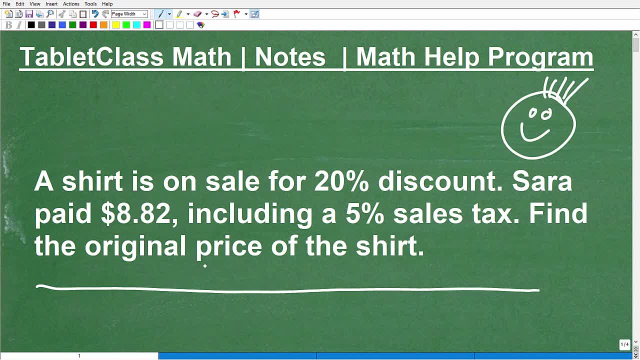 okay, I see how you're getting your answer. you need justification. that is clear. you know your answer needs to be supported, if you will. so I'm going to talk about the general steps to handle word problems here in a second, but first let me quickly introduce myself. my name is John. I'm the 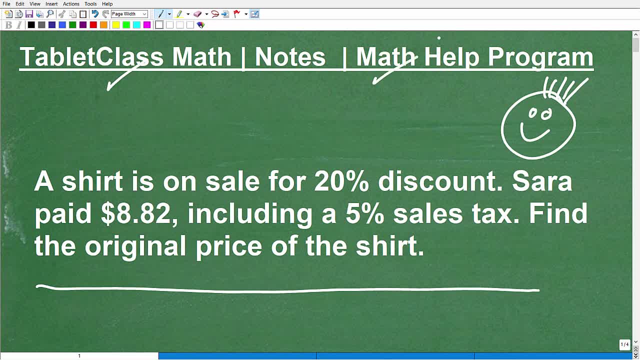 founder of tablet class math. I'm also a middle and high school math teacher and over several years I've constructed what I like to believe is one of the best online math help programs there is. of course, that's a pretty bold statement. I'll let you be the judge of that if you're interested you. 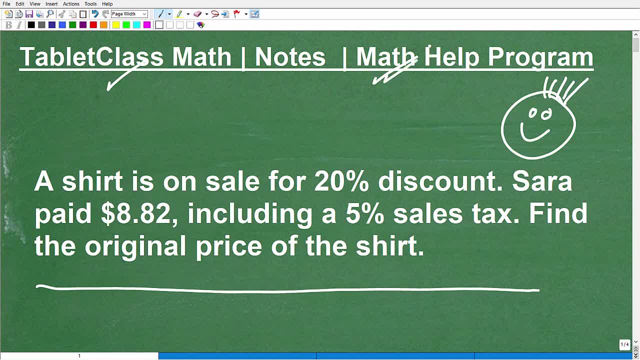 can check out my math help program. I've followed the link in the description of this video, but basically I have a hundred plus different math courses, ranging from pre-algebra, algebra 1, geometry, algebra 2. I'm going to be launching pre-calculus here, uh shortly. very excited about that. all my courses, literally. 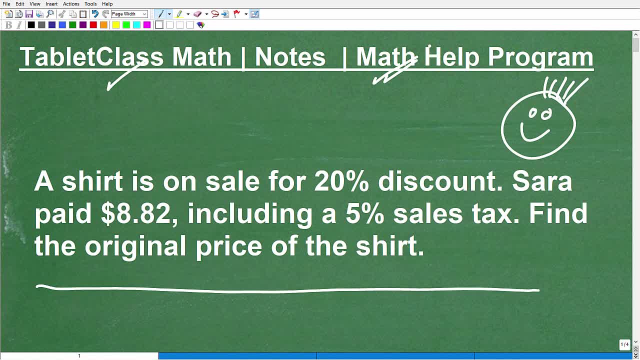 take me years to construct because i don't do quick little tutorial videos. when i teach i try to get my students to be absolutely masters and the skills, the topics of that course. okay, if you're looking for quick little tutorials, you know you might want to check out. you know, keep subscribing. 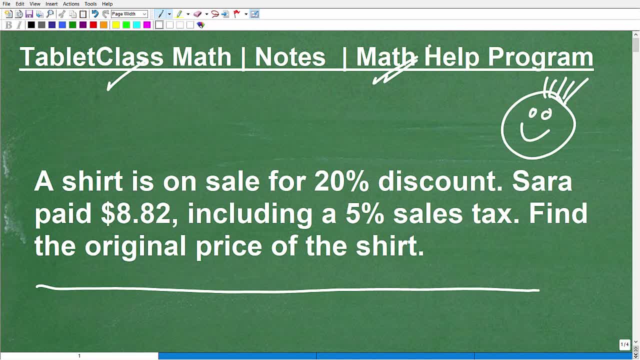 to my or become a subscriber to my channel if you like my teaching style. but if you really want to know this stuff, then my courses are extremely comprehensive, but i also do a lot in the area of test preparation. so if you're preparing for an exam like the ged sat act, uh, maybe the accuplacer 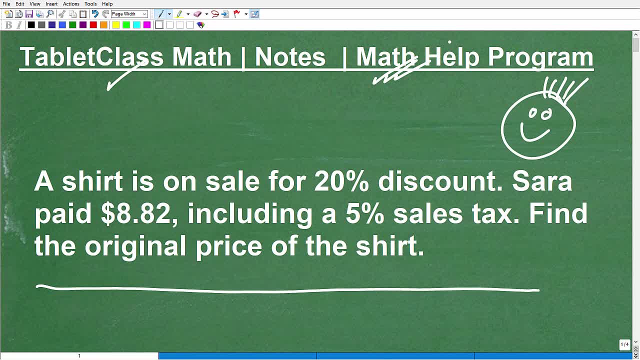 clep exam, uh, teacher certification, nursing entrance- uh, there's a ton of reasons. uh, people need to know math- okay, outside of a math course, because you know. let's say teacher certification. uh, someone goes: oh my goodness, i want to become an elementary school teacher. i have to know a lot. 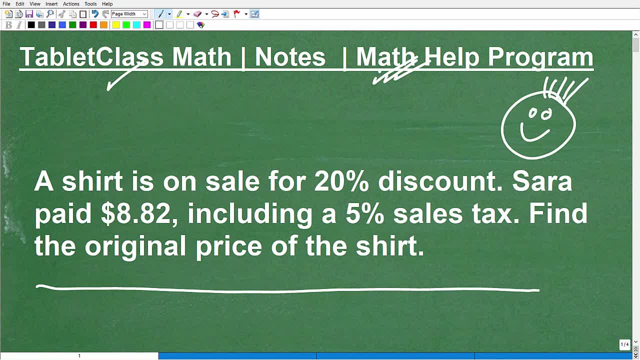 of high school math. so now they have to know a lot of high school math. so now they have to know a lot of high school math. so now they have to go back and relearn stuff. so i have lots of great test preparation, test preparation courses now. uh, if you're interested, just go to my site check. 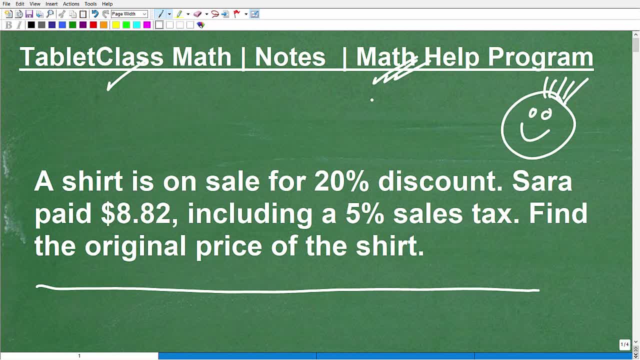 out my full course catalog. if i don't have what you need, drop me a line and i'll give you my best guidance. um, i also work a lot with independent learners like homeschoolers- i have a great homeschool learning system- and then obviously, help those of you who are just struggling in. 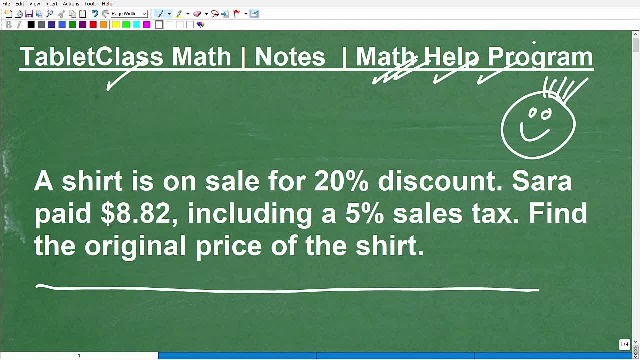 your math class okay, so i could definitely help you out, but one thing you need to be doing to help yourself out- and this is over decades of teaching mathematics- that is to take great math classes and to take great math classes and to take great math classes and to take great. 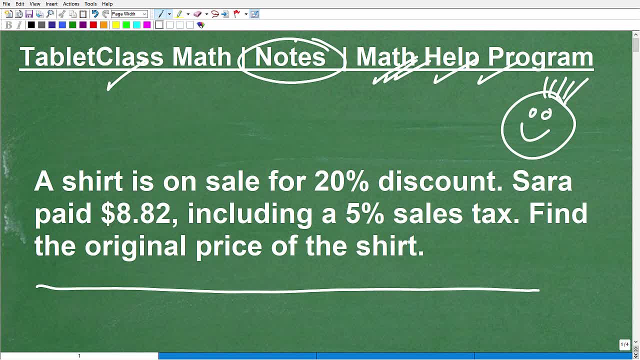 math notes. you're here at this video, uh, to learn about word problems, okay, or this particular word problem, but let's just make sure you are, you know, really doing the most critical thing to learn math and that is to take great math notes. so, over decades of teaching math, uh, just it's apparent. 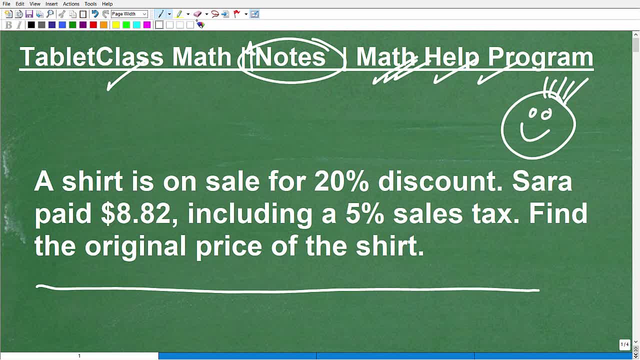 to me, it's like a principle of the universe that those students who take great math notes almost end up looking like this person at the end of the year, and the reverse is true. those students who, um, you know, did what i did back in the 1980s, which was: 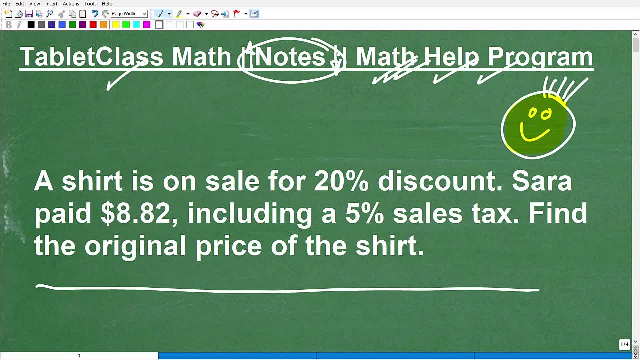 talk to my friends, do my, do anything but listen to the teacher. okay now, if i had a cell phone back in those days, i would have been like real trouble. i don't even know if i would have graduated, but um, of course, uh, cell phones did exist in the 1980s, but they were like huge and there was like 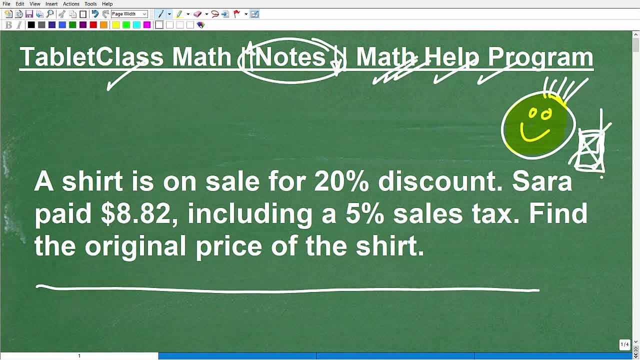 no internet access and no texting, and it cost like ten thousand dollars, some ridiculous amount. so you know- uh, luckily for me, you know i didn't have one of these. but you out there, you have a cell phone and what do we do? we constantly look at our cell phones. 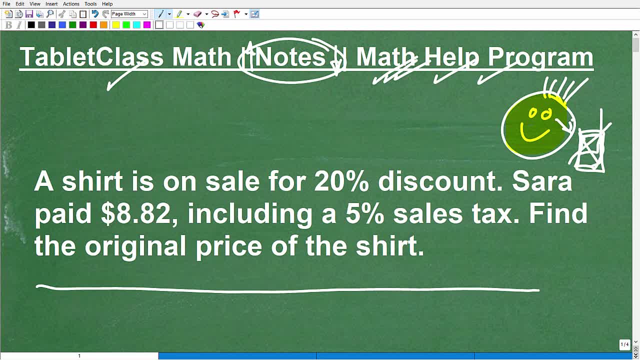 uh, so you have to stay focused and engaged. there's too much information, uh, in mathematics. okay, you're going to miss it, and the only way you're going to, you know, stay focused and engaged is to be engaged in activity, and that is taking notes, and taking notes is all about remaining focused, right that? 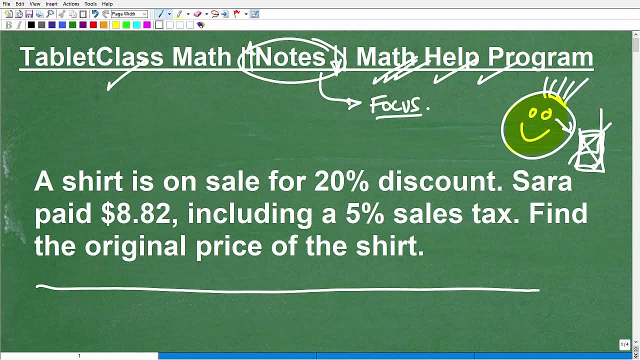 is the key to learning anything. so really look at your notes and take an honest assessment. hey, are my notes really good? not good, i'm talking about absolutely like outstanding. that's what you want to strive for. so, as you're making these improvements, i actually offer detailed, comprehensive math notes to include pre-algebra. 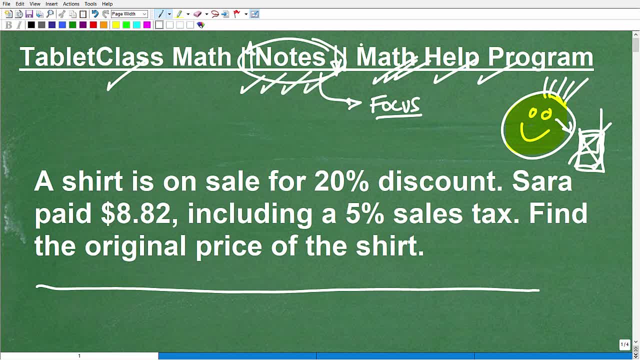 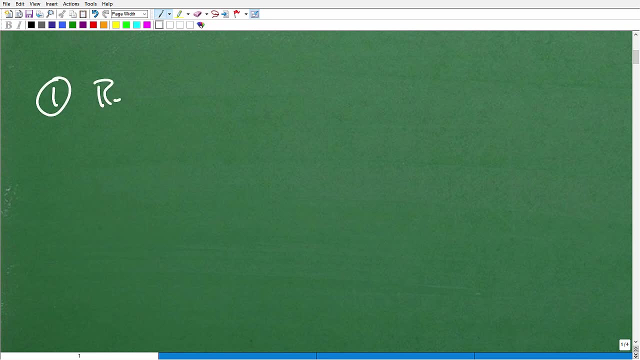 algebra 1, geometry. algebra 2 and trigonometry. you can find links to those notes in the description of this video. okay, so, uh, now we're going to get into this word problem, but let's just quickly review the basic steps to any kind of algebra word problem. so the first thing is you want to read the. 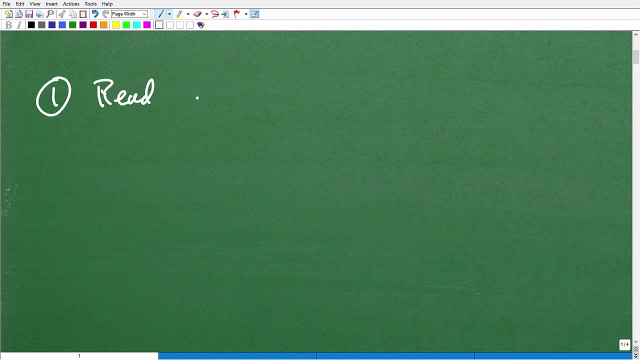 problem and you're probably saying: okay, mr youtube, man, uh, that's like obvious. okay, read the problem. hello, please tell me i didn't watch your video for me to tell you how to uh, that i need to read the the problem. well, what i mean by that is i need to read the problem like five times or more. 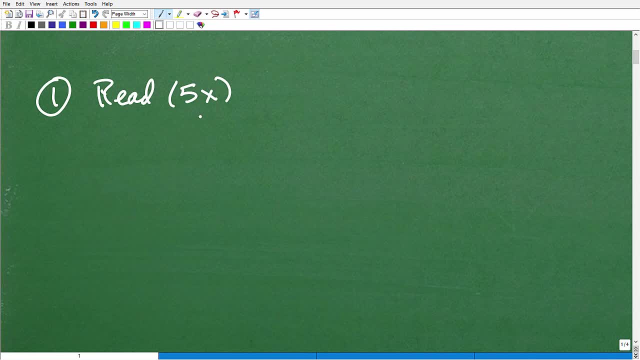 okay, so read, reread, read. don't read it once, because what i'm trying to get at? you cannot read a word problem one time and then just start doing work. okay, you have to read it, get a feel for the problem, read it again and just kind of keep rereading, pulling information out of the 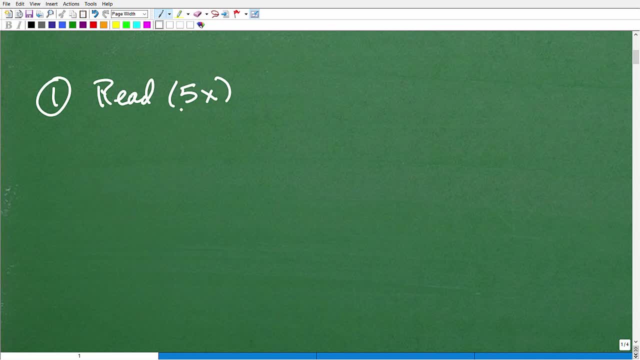 problem. so this is the first thing that you need to kind of have in mind- is you're going to have to be able to read your problem multiple times through that word prompt to pull out information, so don't just try to read it once and then do the problem. the second thing is create some sort of 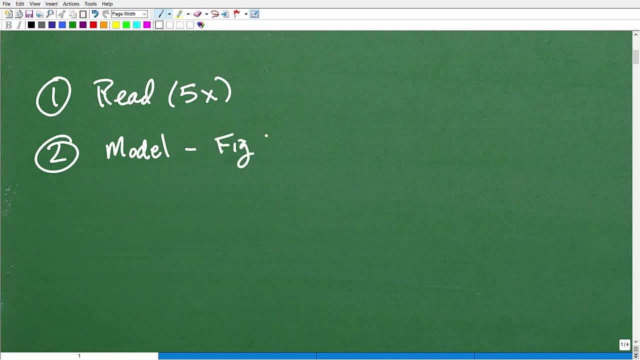 model. okay, now, what i mean by that. it could be some sort of figure, some sort of sketch or a table, some sort of um, basic formula, uh, some, any kind of thing that can help you kind of model the information in the word problem. now, sometimes it's more obvious than others, especially when you're 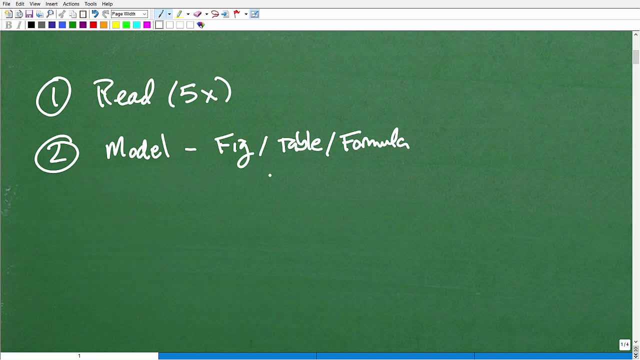 if you're dealing with, like a geometric situation or something else like that and this particular problem. it may not be so obvious, but you want to try to model the best you can, and one person's model could be different from another person's models. the whole idea behind modeling is to help. 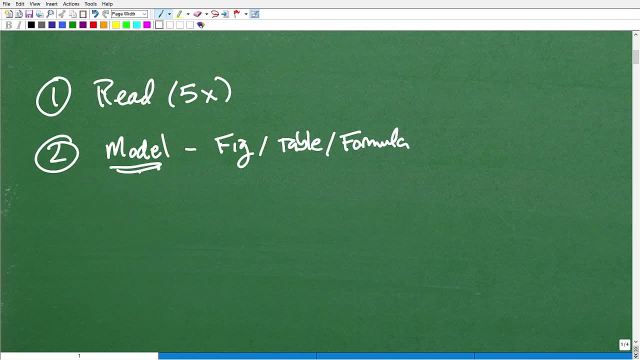 you organize the information and the problem so you can kind of see it better, so you can kind of think about the solution, okay, so you should try to model this and I'll show you all this, all of mine here for this particular problem, here in a second. but I want to want you to stress that. 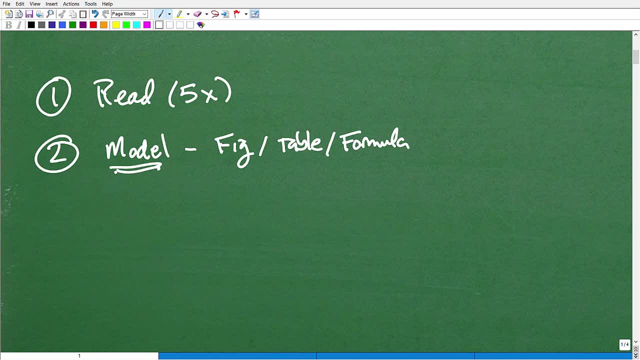 your model can look different than mine, as long as it's logical, okay, it's still very, very good. okay, there's multiple ways to get to the solution of a word problem, more or less okay, at least stylistically. okay, so there's not any one specific way to model. okay, as long as it's logical. 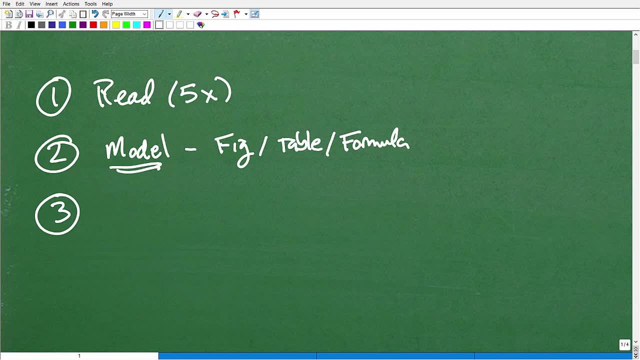 that's the thing you want to strive for. the next thing you need to do is you need to assign a variable, or variable. so we want to say, okay, we're going to let. okay, we're going to let it be right here. okay, so we're going to let it be right here, okay. 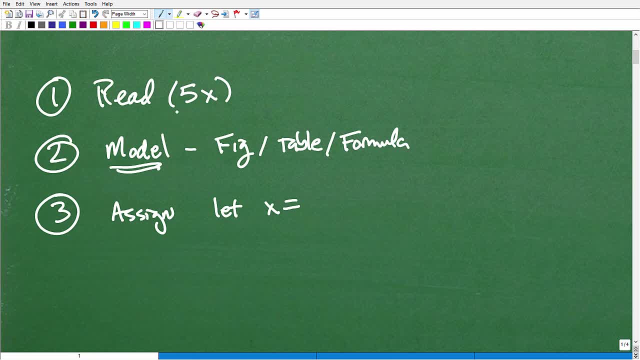 x equal to something. now we're looking for some unknown value. right, it is a word problem and it's the word. the problem is asking you for something that we don't know. so in algebra, we'd like to let you know. variables represent unknown valuables, uh, unknown uh values, excuse me. so we 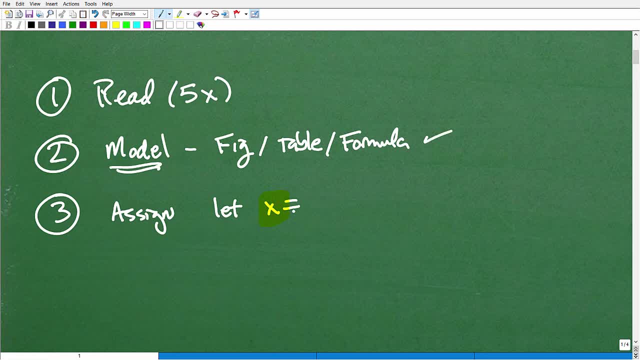 want to start assigning our variables. okay, once we kind of have a model of it, then we're going to be like: okay, we're going to let this x or it could be x, y, it could be multiple variables, it doesn't have to be x, but we want to assign a variable to represent something. now, once we've done that, 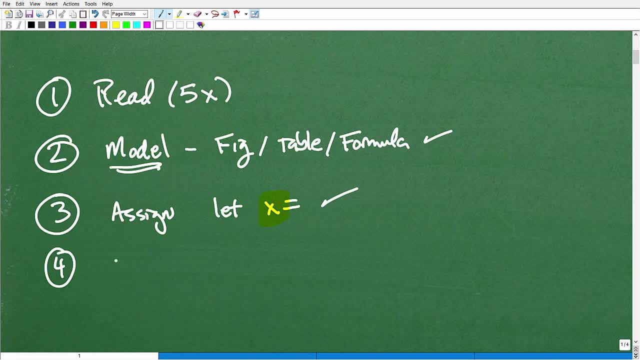 we're going to go ahead and use that variable to try to build an equation. okay, so we are talking about algebra, uh, because in order to solve for that specific variables amount, we need to have it involved in uh in an equation. now the equation is going to be: uh, generally some sort of relationship. 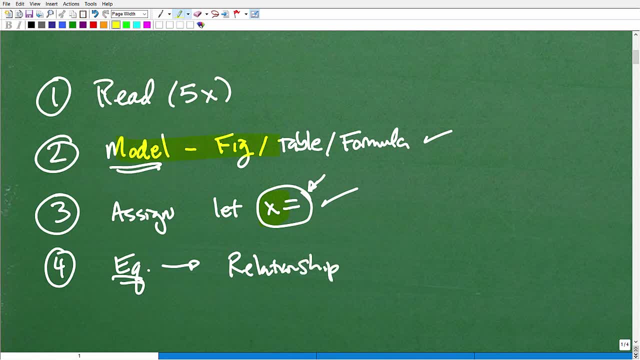 that you're, you can see going on in the problem, And that's where modeling comes in handy. So you look at your model, then you're like, okay, there's some sort of relationship going on here, So I'll use my variable. 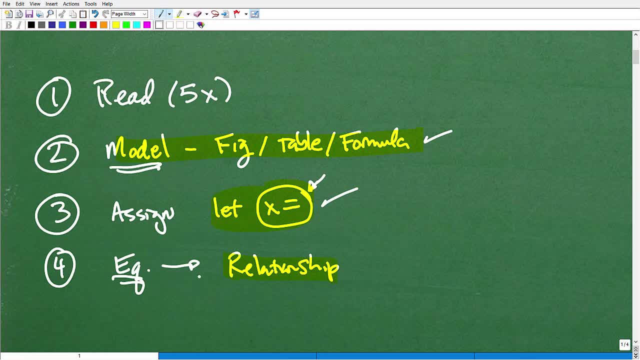 I can see this relationship. So you want to build an equation, an algebraic equation that involves an equal sign and some variables and some numbers, Then the next thing I'm going to do is solve such equations. So we're going to solve the equation from step four. 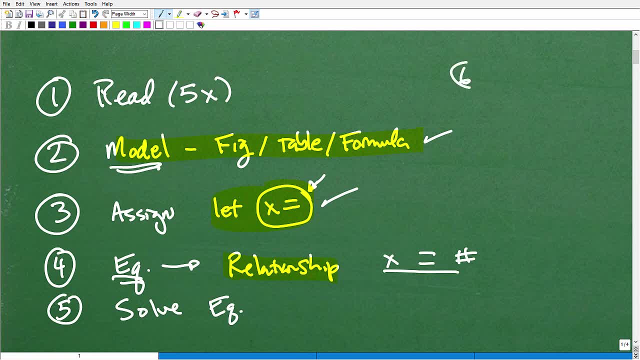 Now this is where a lot of students get themselves in trouble. They're so excited They solve the equation. They're: yay, yay, listen, I got the answer, Mr Teacher. Here it is. Then they end up with a sad face because when you solve the equation, 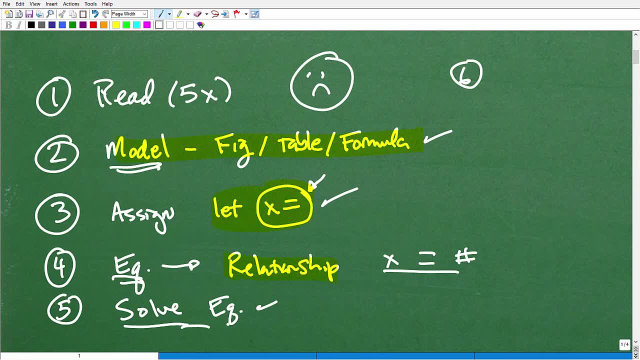 for this particular value. that's not necessarily the answer. So you need to go back and reread and make sure double, triple check. that you may need to take an additional step is what I'm getting at after you solve the equation, to actually answer the question in the problem. 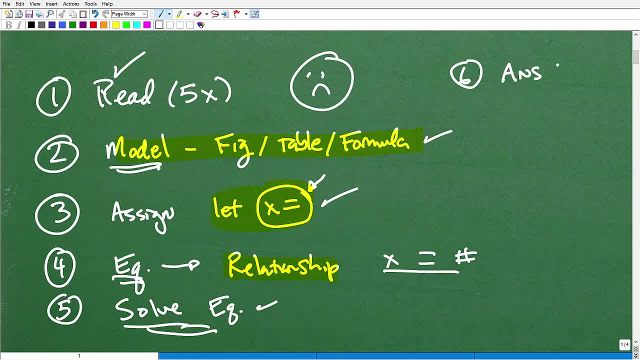 Okay, So that's what we want to do. Our last step is make sure we answer the correct question, And that's not always necessarily the solution to the equation that you have from step four here. Okay, So in algebra, if you follow these general guidelines, 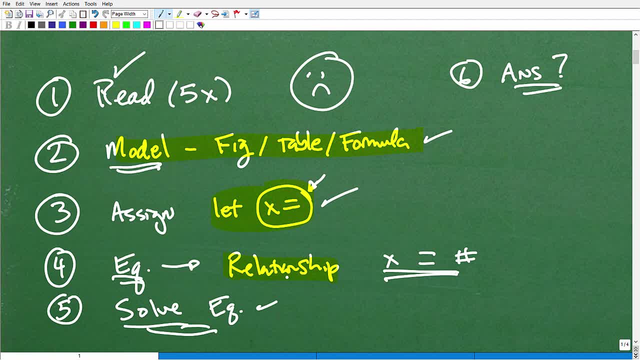 you should be pretty good to go on word prompts. Again, in algebra there's a lot of kind of classic, typical type of prompts and this is one of them. Okay, So if you want to try this problem again without me, 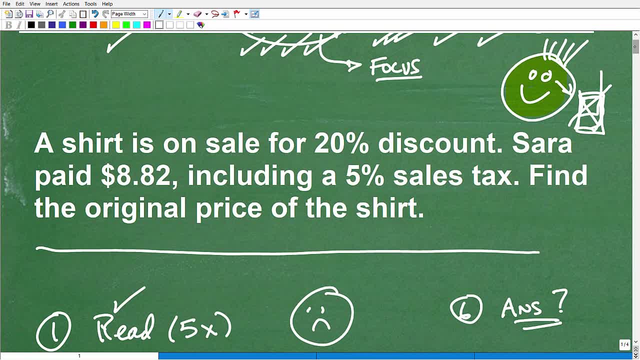 you know, without seeing a solution, here it is, You can pause the video and give it a whirl. now that you have this general guidance, But if you don't want to see my solution, go ahead and keep the video paused, because I'm going to get into my solution now. 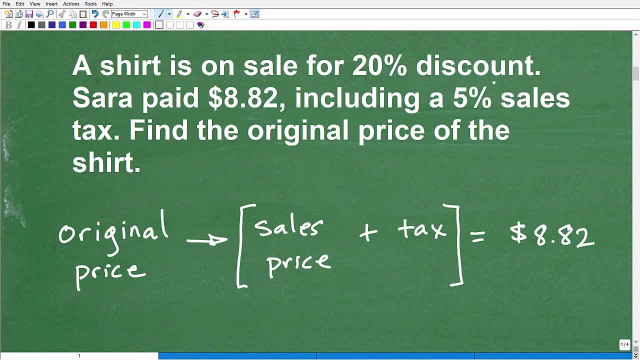 All right. So a shirt is on sale for 20% discount. Sarah paid $8.82, including a 5% tax. Find the original price of the shirt. So that is the problem. Yeah, $8.82.. You know it's pretty, you know inexpensive. 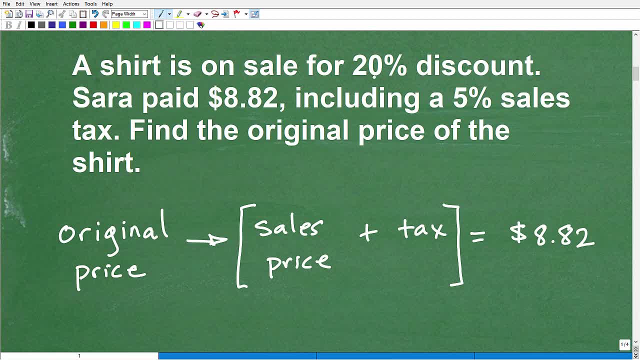 I was going to say the word cheap, but maybe it's a good deal. You know, it's obviously got 20% off. So you know a lot of you are like, wow, $8.82, that's not, you know, listen. 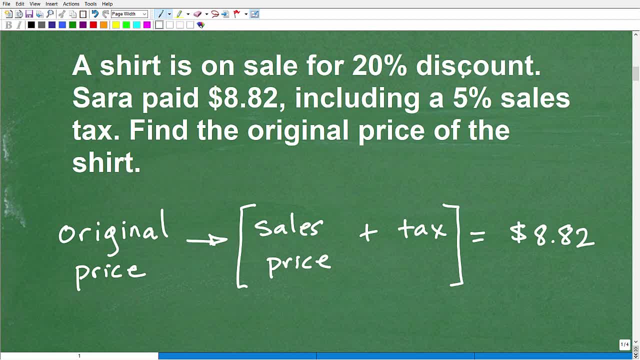 don't worry about that part of the problem. Just it is what it is right, Okay. So let's just kind of get a feel again for the problem. So what is the problem asking? Okay, so find the original price of the shirt. 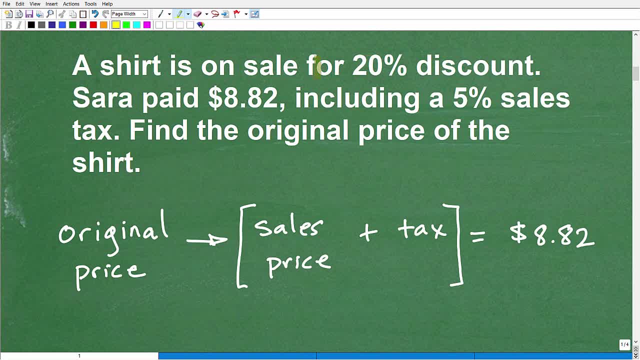 We don't know the original price. We do know that the shirt was on sale for $20.. So if you kind of model out what's going on, we had an original price, Okay. Then that original price was dropped down by 20%. 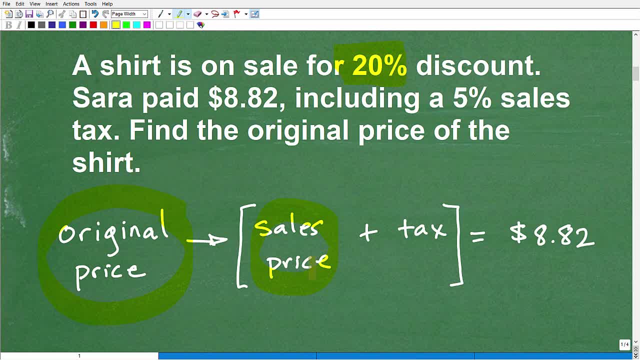 Okay, It was on sale, So we had a sales price, And so what happened was that Sarah paid $8.82.. Okay, So she had the sales price of that shirt Plus she had to pay the tax on that shirt. So this was our total expenses, if you will. 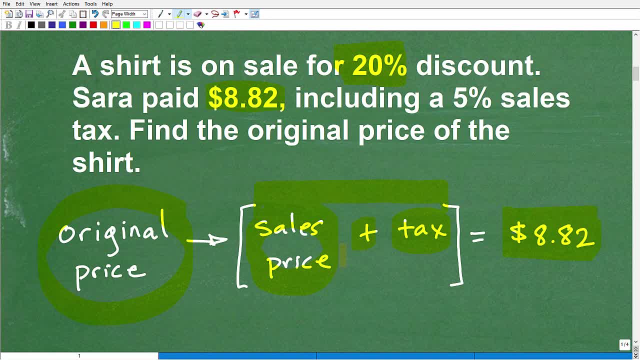 And it came out to $8.. So, conceptually, this is kind of what's going on And the question is asking for the original price, Okay, So the original price was some amount, Okay, And we know that the sales price was 20% off. 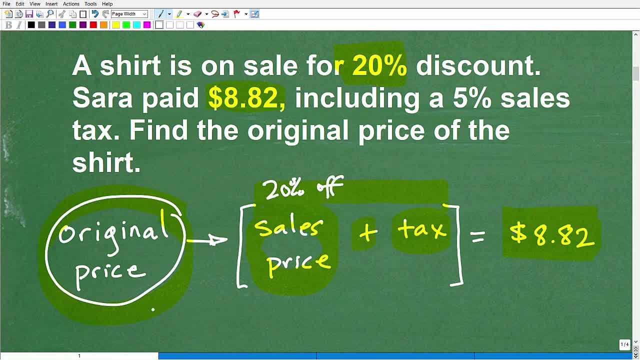 But in terms of decimals it is 80%. The sales price is 20% off, but it's really 80% of the original price. Okay, So if we take 80% Of the original price, that is in fact the sales price, which is a equivalent to a 20% discount. 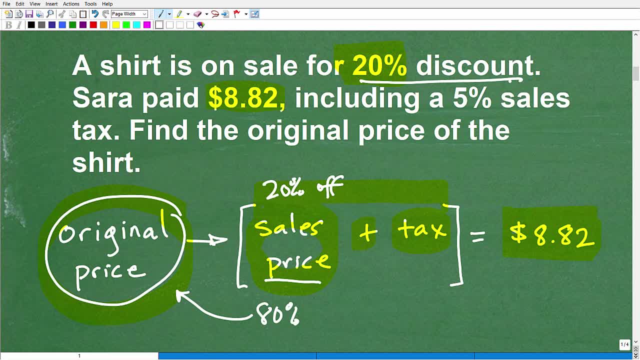 So this is kind of a general model or structure that you kind of keep in mind in terms of the information and the problems and the relationships. So again, we want to find the original price of the shirt, So we need to start establishing some variables here. 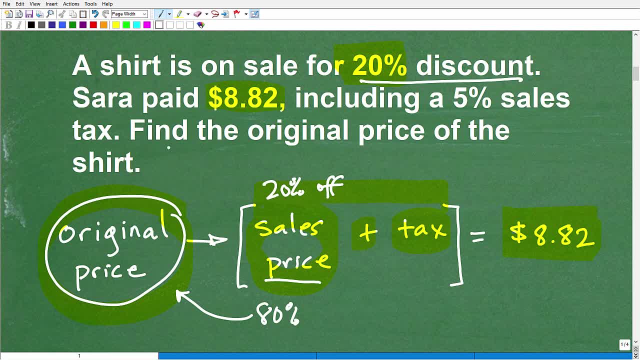 So you know, it's a good idea oftentimes to let our variable represent what we're trying to figure out. So here we want to find the original price of The shirt. So why don't we let X equal the original price of the shirt? 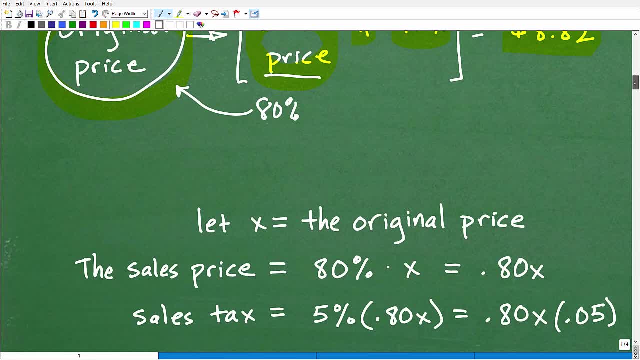 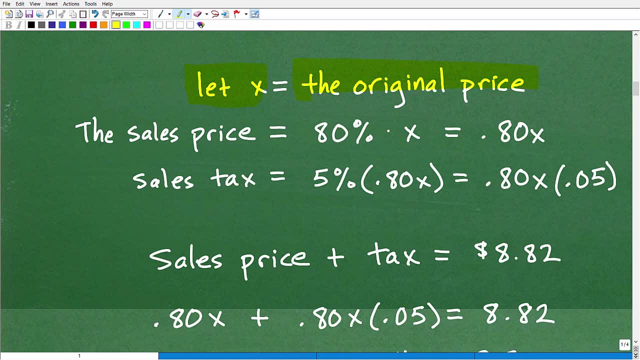 And that's what I've actually done, So let me show you this here. I won't get the work in advance, Okay. So let's let X equal the original price of the shirt. That's what we're looking for Now. the sales price of the shirt: as I indicated, it's 20% off the original price. 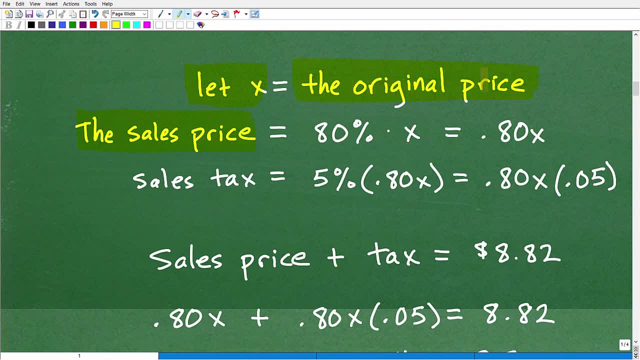 Okay, But it's really 80% of whatever that original price was. For example, if the The original price was $100 and I got a 20% discount, that would be $80.. I would pay $80.. So the sales price is 80%. 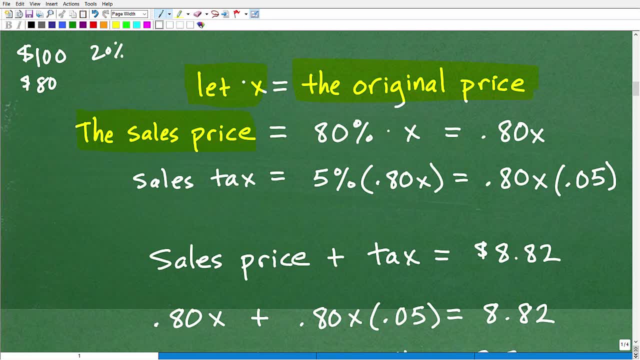 Okay, 80% of that original price, which is X now. Okay, So 80% times X. Now I'm assuming you know about percent. If you don't know about percent, then you need to do a quick percent review. 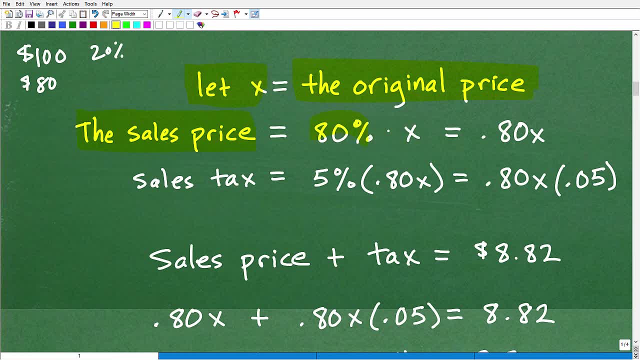 But the sales price will be 80% of the original price. So 80% times the original price, 80% as a decimal And we want to find a percent of a number. We change that percent to a decimal, So that's going to be .80 times X. 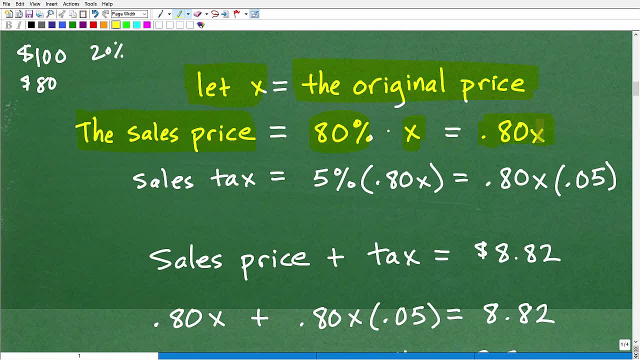 Okay, So the sales price we can represent as .80 times X. So hopefully this makes sense to you All right Now. if you're a little bit rusty on percent, you want to go back and review basic percent, and you're lucky because I have. 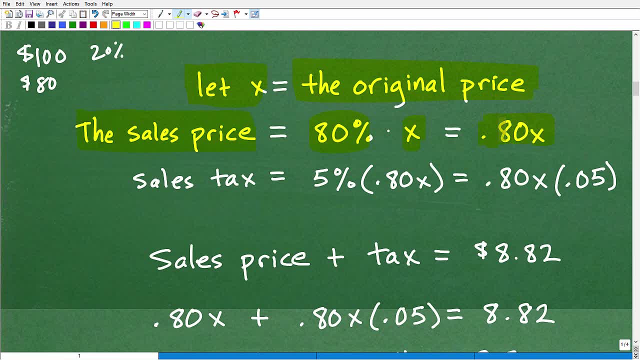 tons and tons of videos on basic percent In my pre-algebra playlist on my channel that you kind of circle back to this problem. All right, So that's the sales price of the shirt, right, 80% or .80 of the original price. 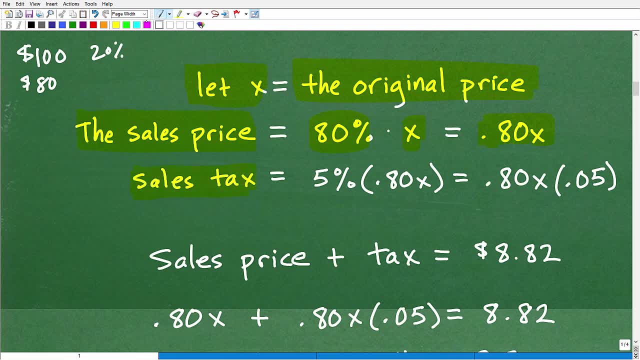 Now the sales tax. Okay, When you go check out at the checkout counter, right You have your tax and that's everyone's favorite Work. problems and taxes are probably everyone's favorite topic. Now, I know a lot of you are laughing at that. 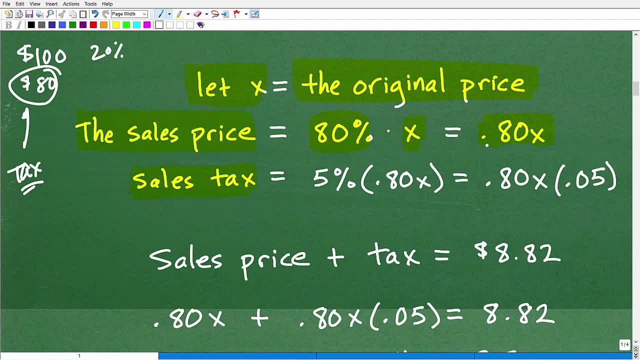 But anyways, you got to pay this tax, right? So you have 80% or .80 X. that's the sales price. Now we're going to pay tax on that sales price, that sales tax. And we were told: okay, let's go back up to the prom. 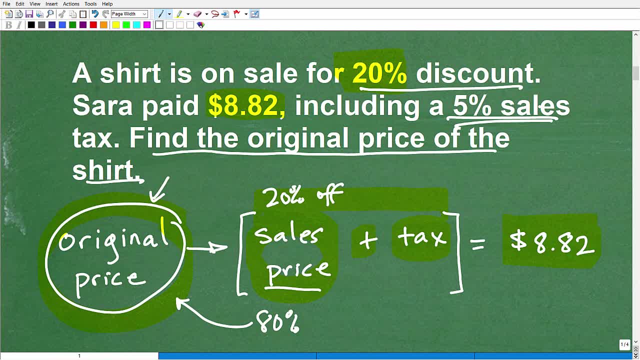 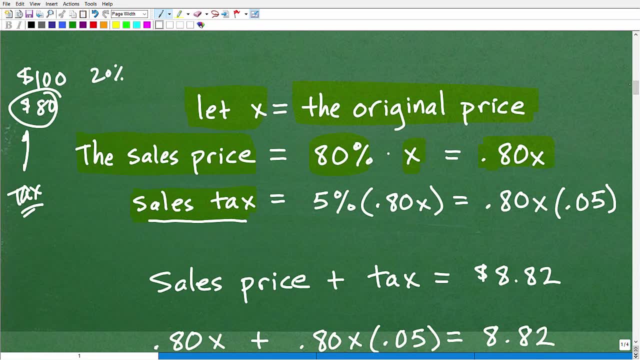 that the sales tax is 5%. So we're rereading the problem, kind of circling back. Of course I'm doing this. you know I did this work in advance, but you would have to go back and keep pulling this information out. 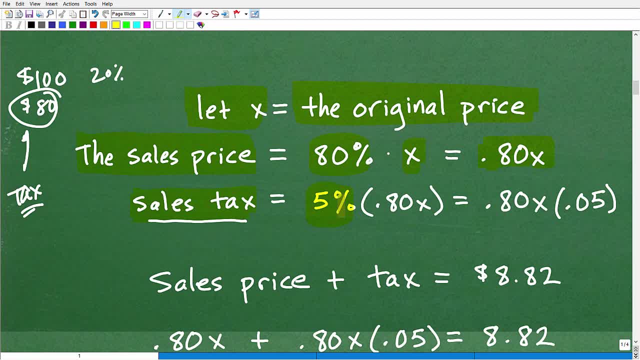 So what's the sales tax? Well, it's going to be 5% off the product, the price of the product that you're buying. So the price of the product that I'm buying is .08 X. It's the the sales price of the shirt. 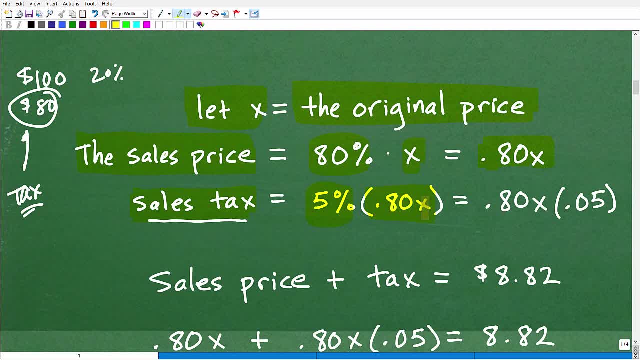 Okay, So this is what I'm actually paying for the shirt: .80 X or 80% of that original price, But now I got to get the additional 5%, So 5% of that sales price is going to be my tax. 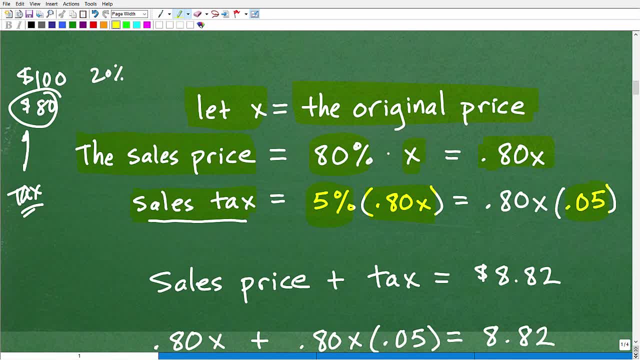 All right, So this is again. I take that 5%, write it as a decimal, So that's .05.. And I'm going to multiply that by this .80 X. Okay, So before you continue on with this problem, really make sure you understand this layout. 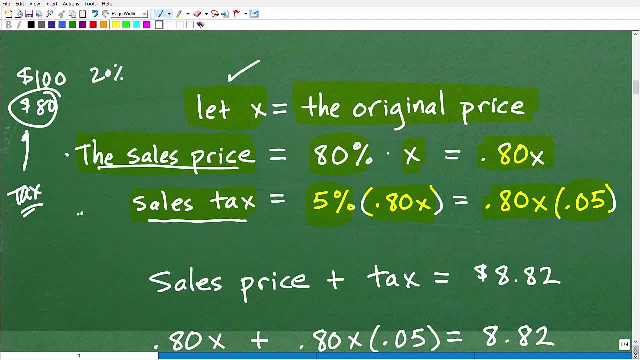 Okay, So we have signed our variable and we're kind of structuring things like this. Now it's time for us to kind of build an equation, Okay. So this is where our model kind of comes into play. Okay, This kind of modeling. 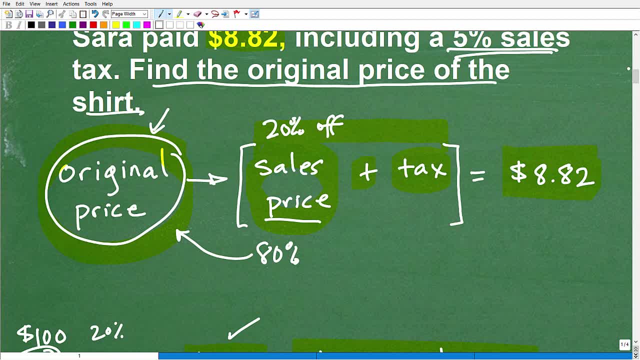 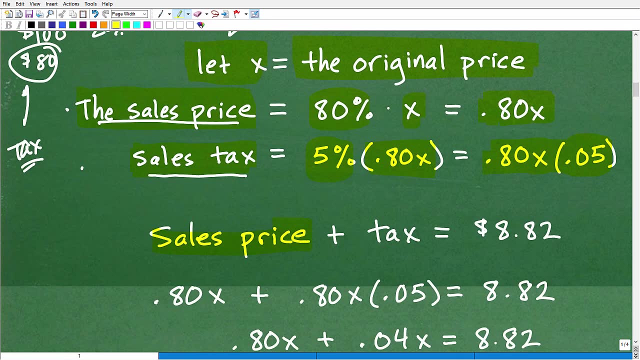 And this is just, you know, like some sort of organized kind of information, Organizing techniques. Okay, It could be graphic, graphic organizer, It could be something just kind of right out, But this model is effectively saying this: We have a sales price. 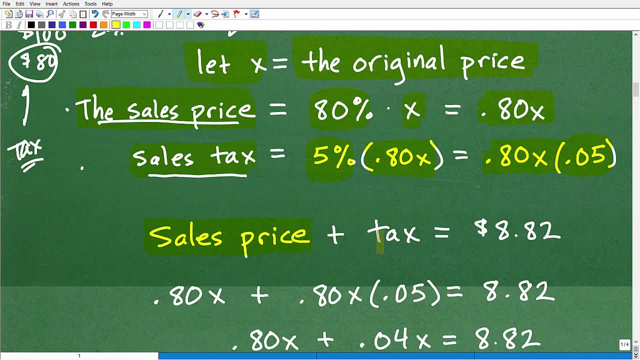 Okay, Sarah has to pay for the sales price of the shirt plus the tax and her total bill, Okay, At the checkout counter is $8.82.. Okay, So now we have an equal sign involved and we can build an equation, because I know the sales price of the shirt. 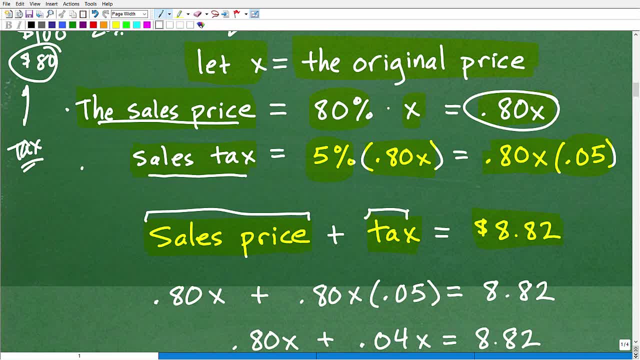 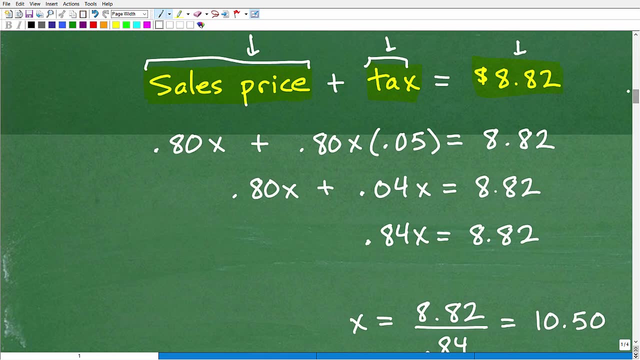 It's this .80 X, and I know the tax now of that shirt, That's going to be .80 X times .05.. So I just plug those in here and I can build myself a nice algebraic equation. So let's go to do that now. 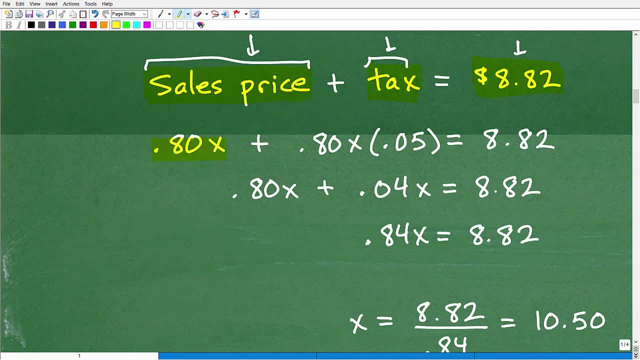 All right, So a sales price of the shirt is .80 X, The tax is .80 X times .05.. Right, 5% of that sales price of the shirt. So now I'm like, okay, I got to figure this out, but let's just finish it out here. 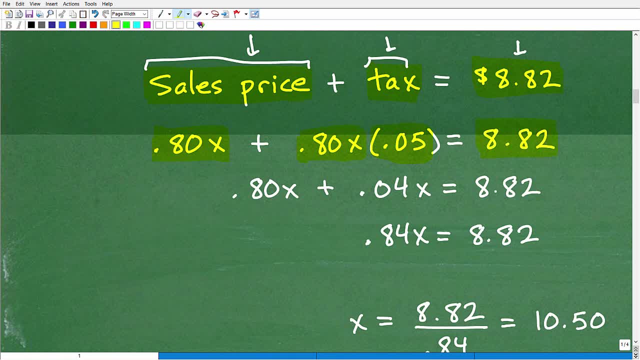 I got $8.82.. So I can just drop the dollar signs. Let's just figure out what X is equal to, right here. All right, So .80 X. at this point Let's just say that you know your basic algebra equation solving skills. 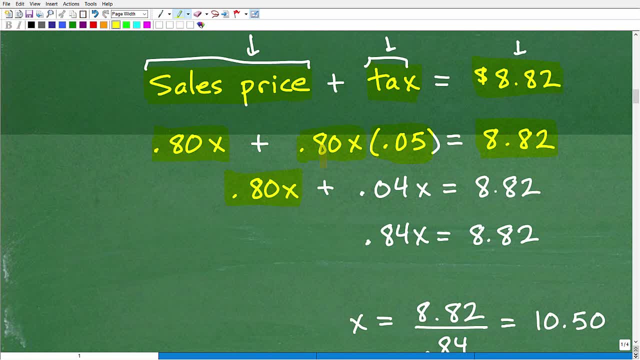 Now, if you don't- that's another thing- you need to go back and review. So .80 X times .05, you can use our calculator: .05 times .80 be .04 X. So I have like terms here. This is X, This is X. 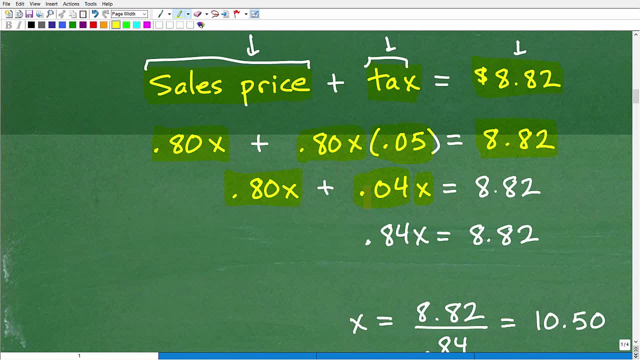 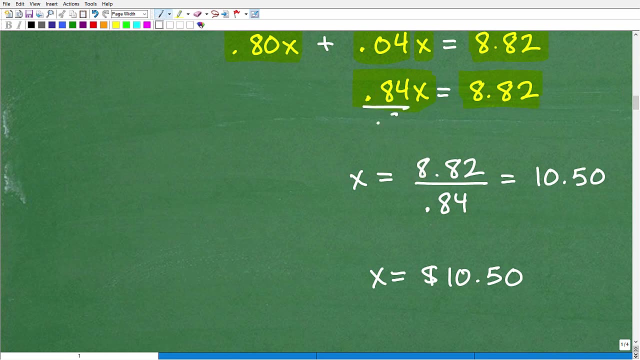 I can combine these, So .80 plus .04 X is going to be .84, X And that's going to be equal to 882 or 8.82.. And to solve for X, I simply divide both sides of the equation by this .84.. Okay. 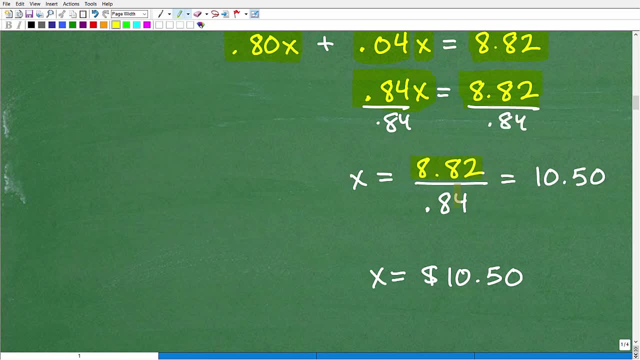 As you can see I did here. So 882 or 8.82 divided by .84, X is going to be equal to 10.50.. Okay, Now, what does that mean? So X is equal to 10.50.. 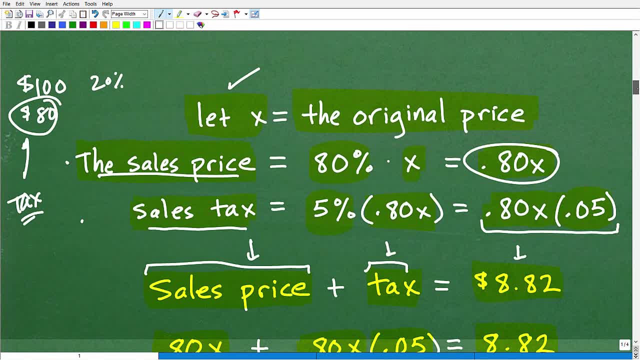 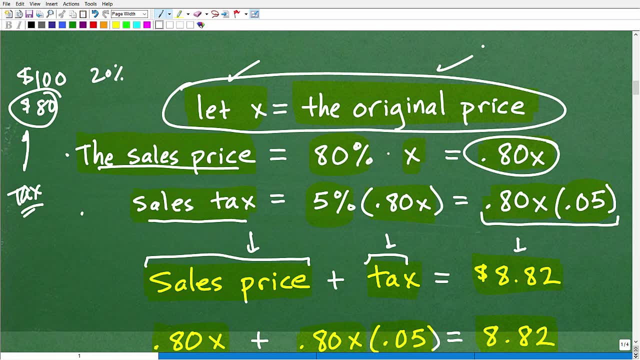 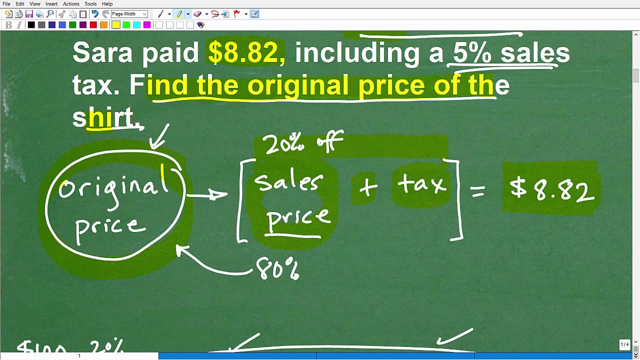 Well, you got to circle back here And remember we said we're going to let X equal to the original price of X. Okay, That's what I just solved. for What is the question asking again? It says: find the original price of the shirt. 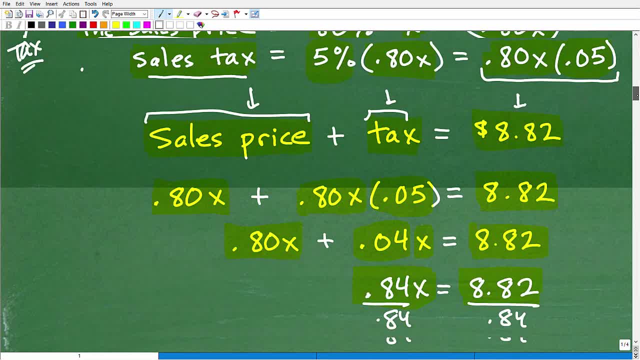 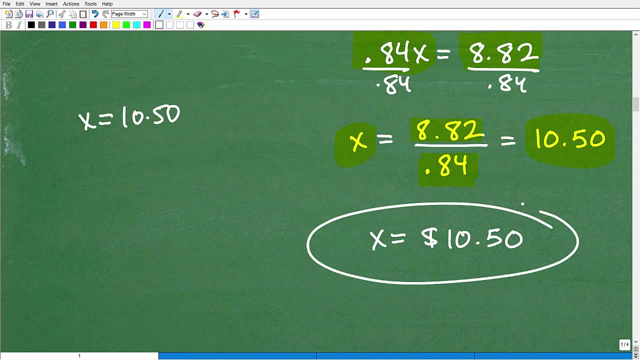 Okay, good, So that was X. So now down here, if we solve for X, we're actually answering the question. So the original price of the shirt is $10.50. And that's it. Now, if you got this problem right all on your own, I just must give you a happy face. 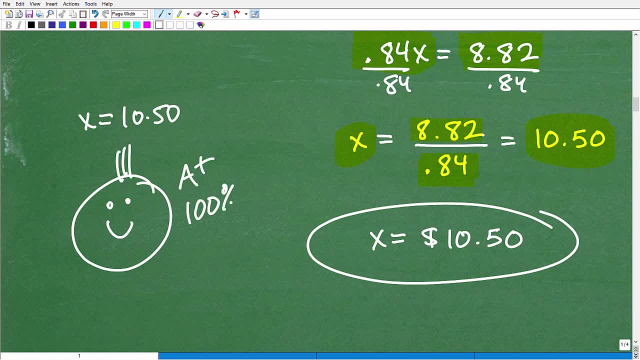 with a mohawk and a plus a 100%. I'm going to give you three stars because this was a pretty, you know, intermediate level problem. Okay, So I mean, if you were in my class I'd be like, wow, you're really good at word prompts. 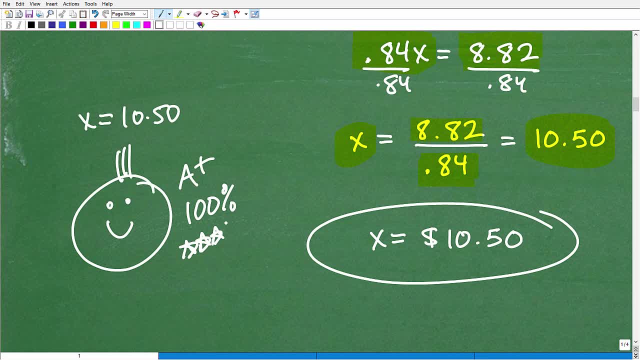 Matter of fact, just take the textbook, go home. I'll see you next year. I said you must be watching that guy on YouTube because you did an outstanding job. All right, So look, here's the deal. You want to get better at word prompts. 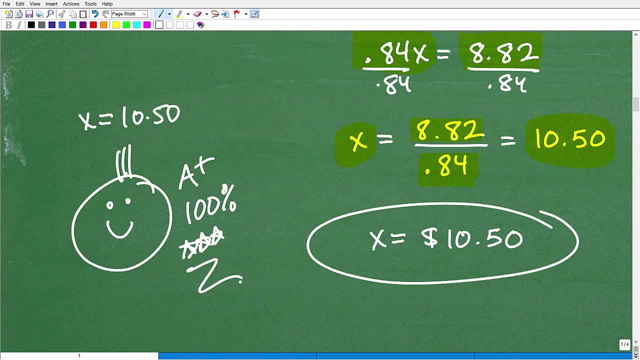 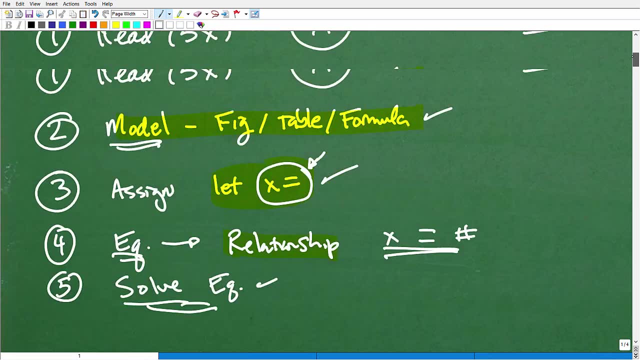 There's one way to get better at word prompts, That's to do more word prompts Practice. It's one thing to watch me do The problem, it's a whole nother thing for you to do the problem. But as you do the problem or you watch me do the problem, you have to ask yourself: 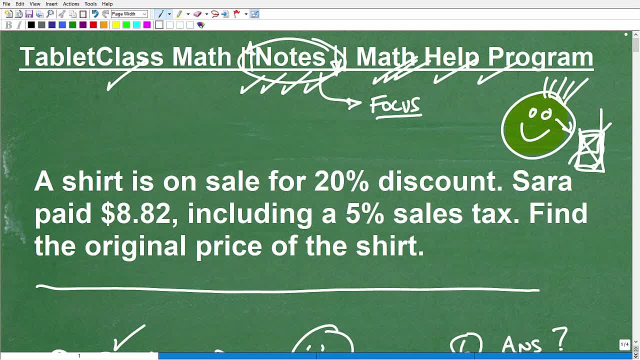 you know, do you understand all the different skill sets involved? And that's where you have to do the hard work. Oh, okay, I was a little confused about percent. Then review percent or like: oh, I'm a little confused on solving equations. 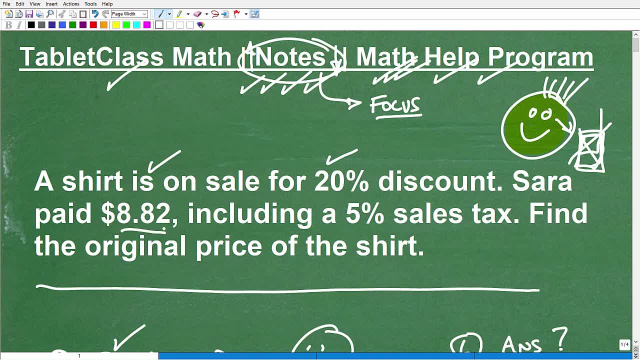 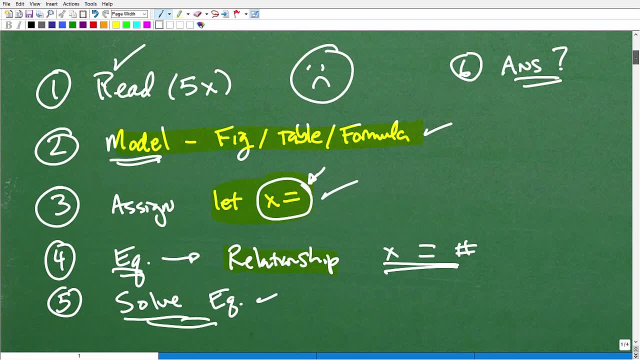 Then you got to review equations. Remember, word prompts are an application of all these skills and they all kind of tie in together. But again, generally speaking, in terms of algebra, these are going to be the main steps that you're going to want to follow. 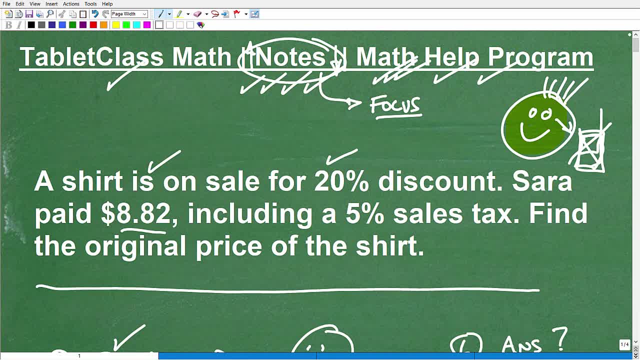 Okay, so we're going to wrap up this video. If you like this video in some way, if it helps you out, please consider smashing that like button. That helps me out. And if you're new to my YouTube channel, please consider subscribing.